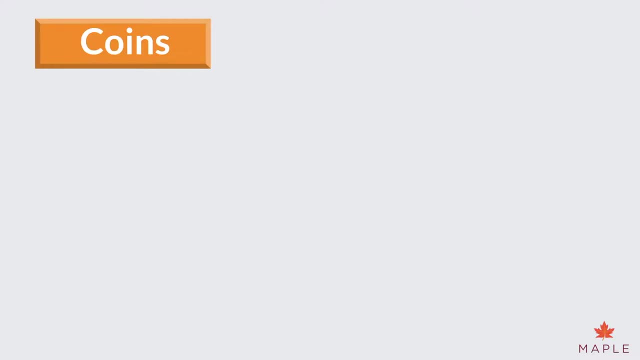 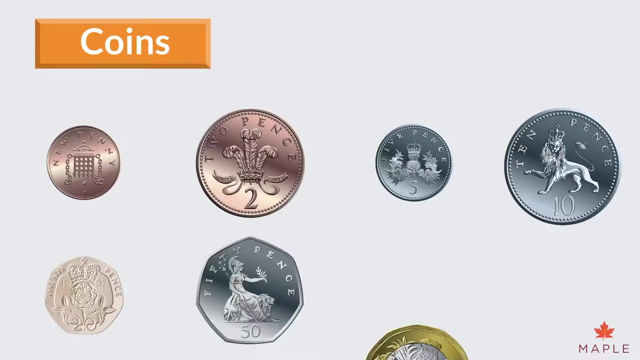 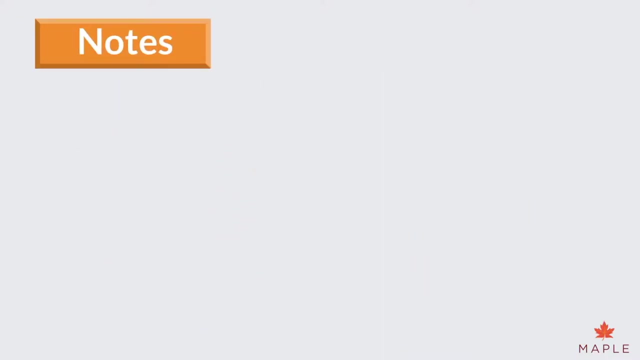 We have the following coins: 1p, 2p, 5p, 10p, 20p, 50p, 1 pound and 2 pounds. We also use notes. The 5-pound note, 10-pound note and 20-pound note are the most used, but you may occasionally see a 50-pound note. 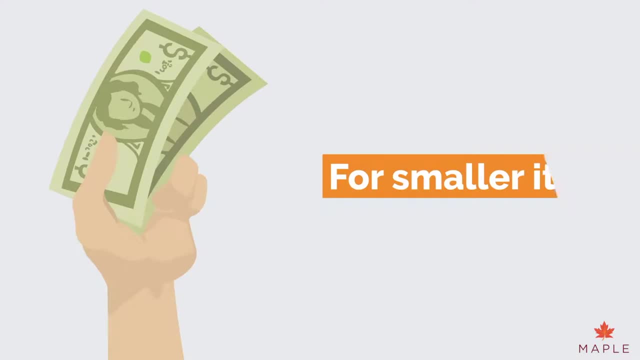 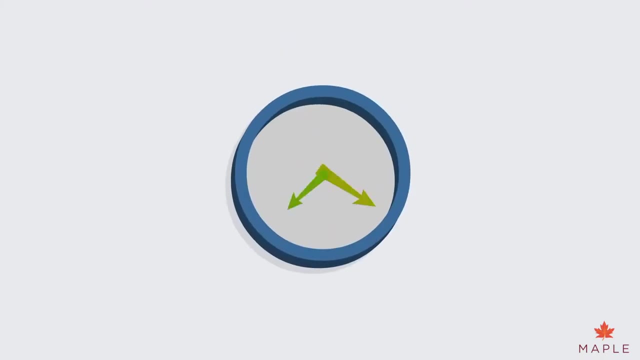 For smaller items, we usually use cash. In maths, working out your change is useful. Most of the time you will need to use subtraction or addition. Have a look at these examples: D'Arcy received 100 pounds from her grandma, 40 pounds from her uncle and 25 pounds from her aunt. 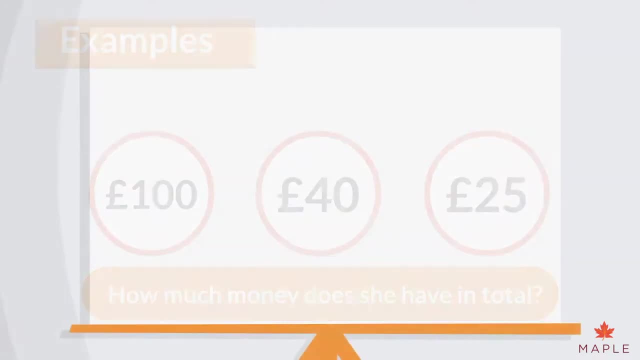 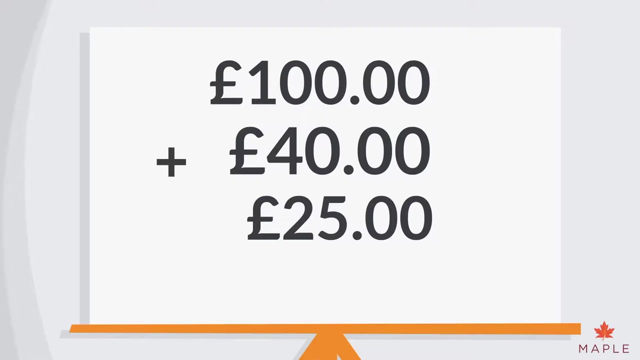 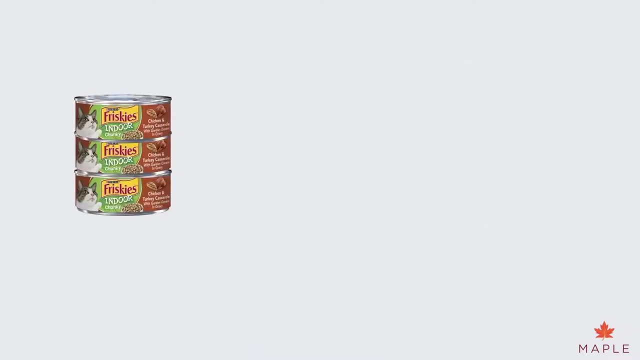 How much money does she have in total? We simply line up all the digits carefully in a column and add them together. D'Arcy has 165 pounds. Lucky girl, Mrs Tibbles, buys three tins of cat food for £1.. 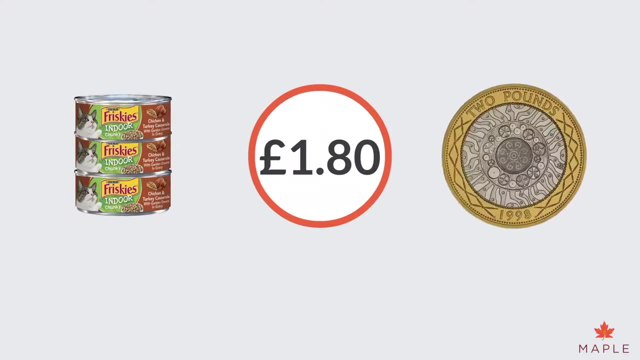 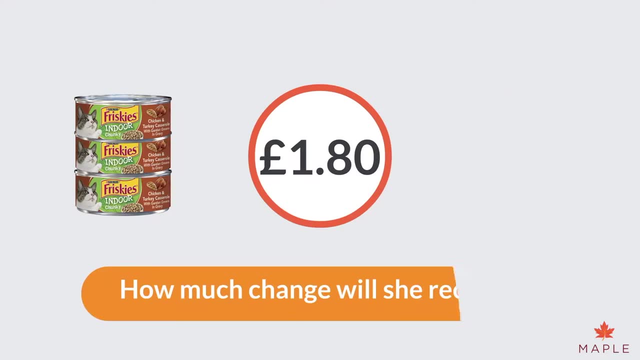 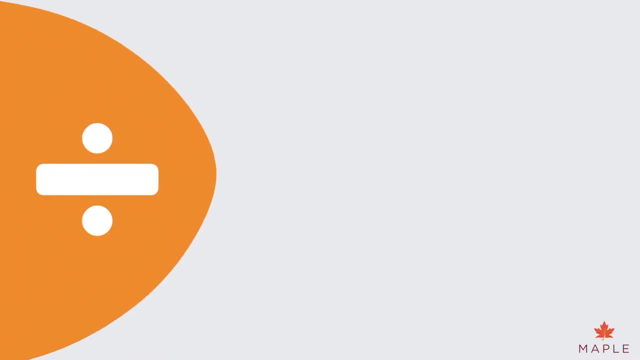 She has £2.80 in total. She pays with a £2 coin. How much change will she receive? This is easy peasy: lemon squeezy. We subtract £1.80 from £2, which is 20p. We can also divide and multiply money too, just like normal numbers. 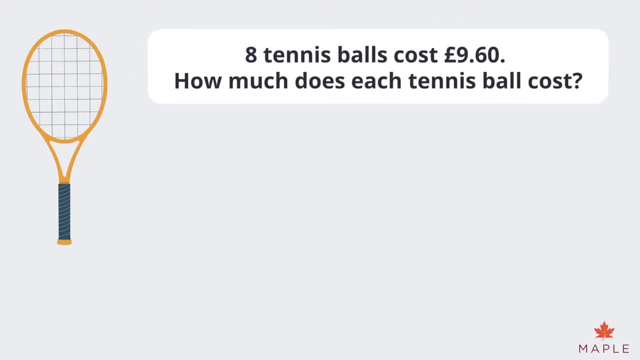 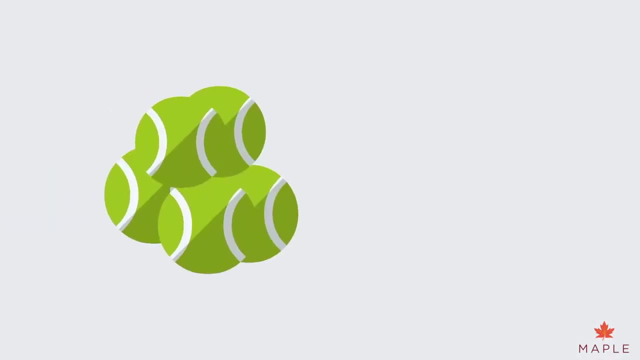 Eight tennis balls cost £9.60.. How much does each tennis ball cost? We can use notes. We can also use division to divide £9.60 or 960p by 8.. Each tennis ball must be £1.20.. 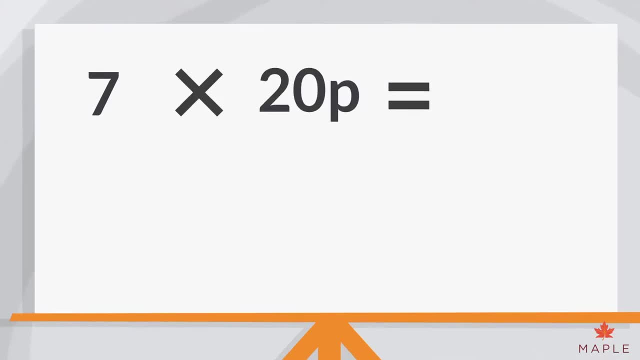 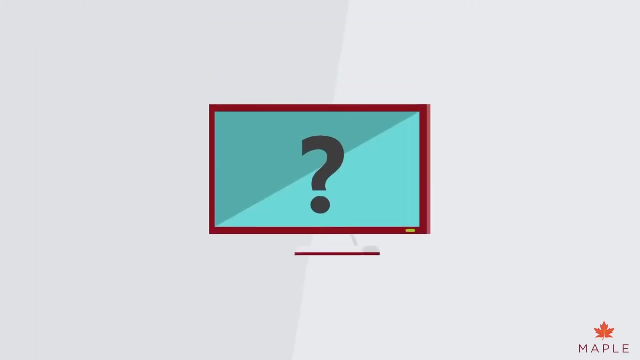 Seven lots of 20p sweets equals 140p or £1.40.. Six lots of three pounds is £18.. Always remember to put the units in your answer. Is your new TV 456p or £456?? There's a big difference.